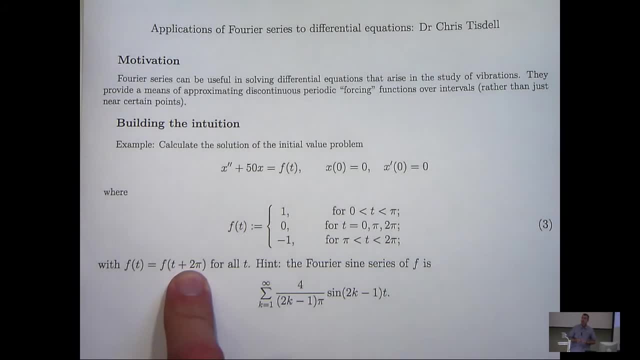 the forcing function is periodic, with period 2, pi. Now the initial conditions may be interpreted as the system starting from rest with zero displacement. Now we're given a hint. We're told that the Fourier sine series of this is going to be 0. And we're told that the 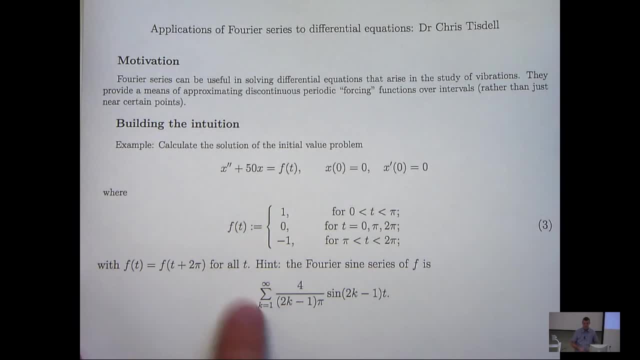 external forcing function. is this series here Now? in fact, I've actually calculated the Fourier sine series of this function in another video, So if you want the details there, you can look it up. But what we're going to do is use this information to solve this differential. 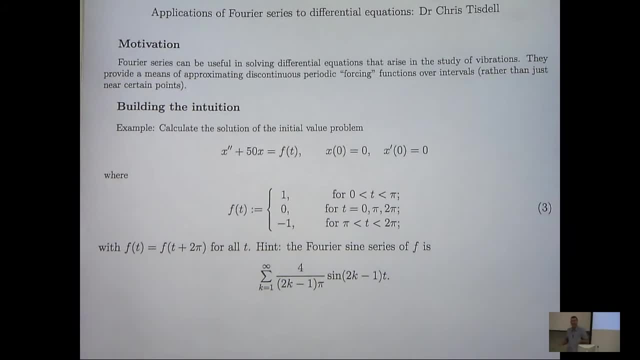 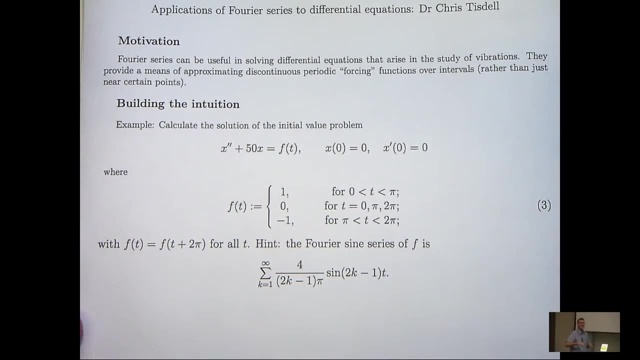 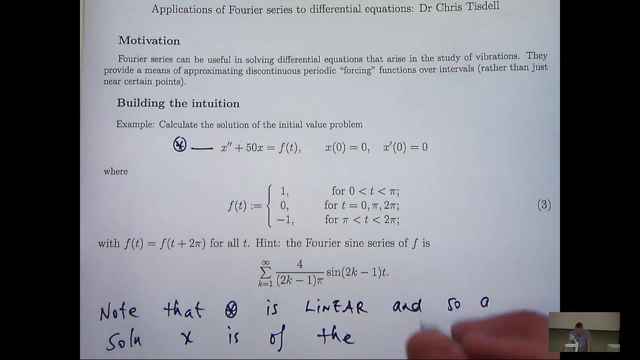 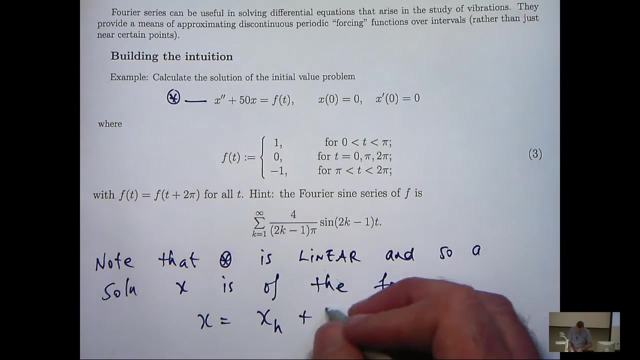 equation. Now I'm going to break it down into a number of parts, And the first idea is that this is linear. So we know that a solution- so let's call this star a solution- x is of the form x equals x sub, h plus x sub. 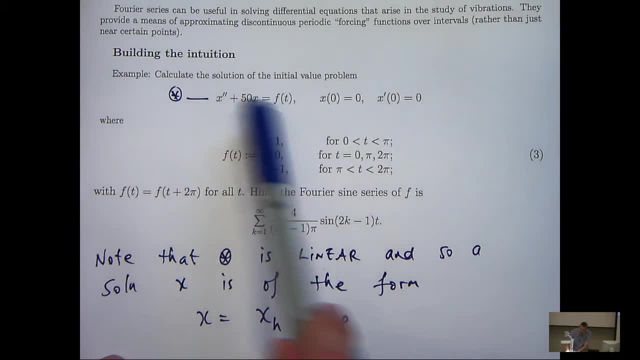 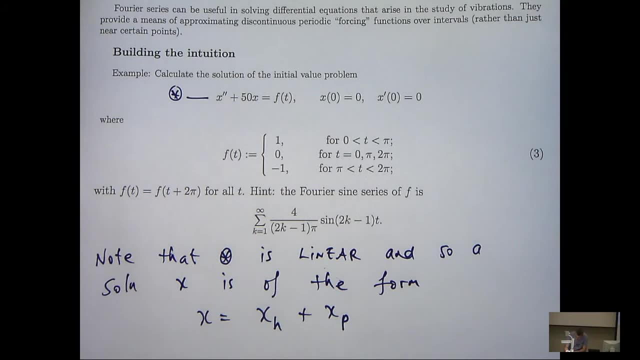 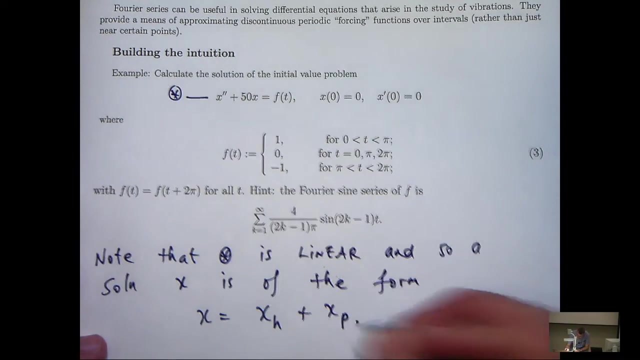 p. Now x sub h is a solution to the homogeneous version of star. So you replace f of t with zero And x sub p is a particular solution to star that we construct Now. x sub h is quite easy to formulate. X sub p takes a bit more work, So let's do. 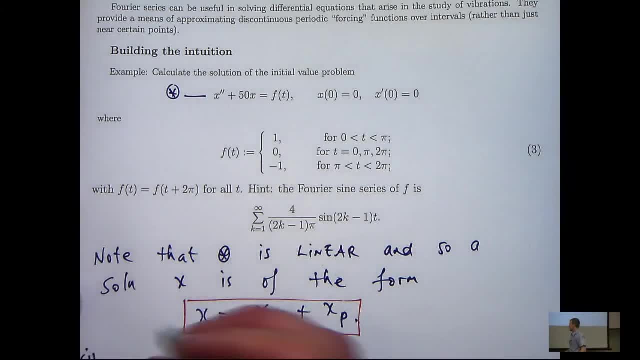 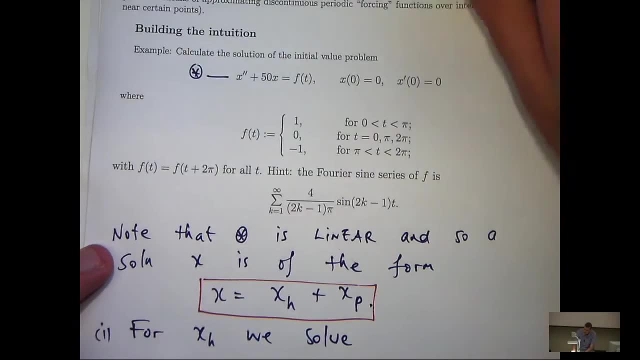 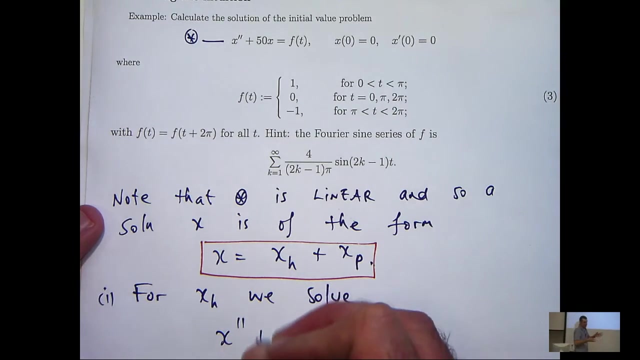 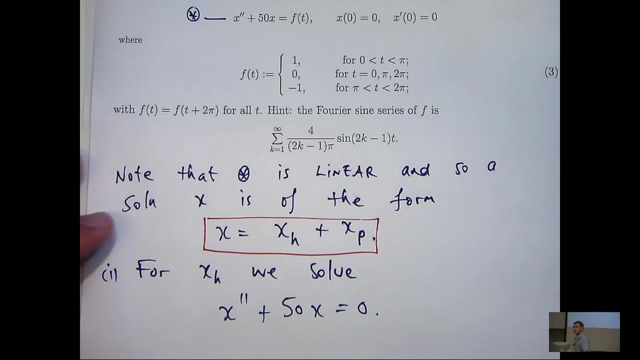 that. So for x sub h, we solve the corresponding homogeneous equation related to star. So we replace the right-hand side with zero. Now you would have seen this in first year. Basically, you look at the characteristic equation associated with this, which is just: 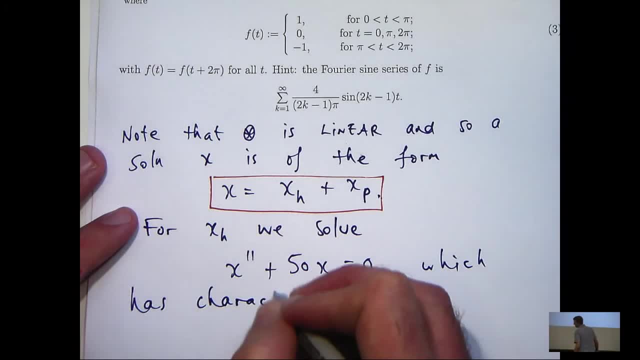 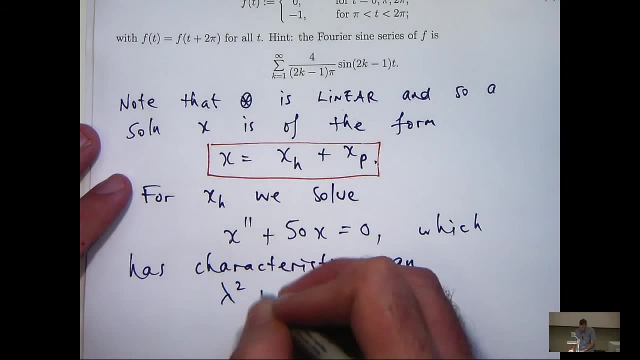 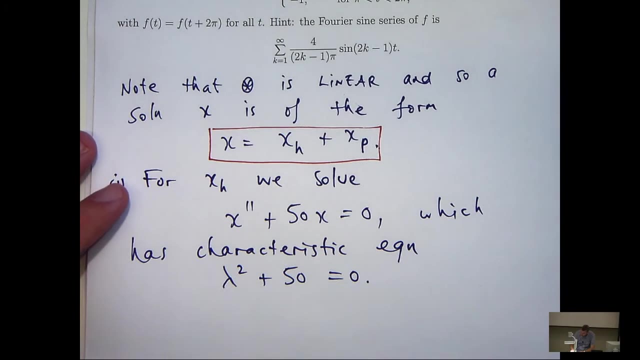 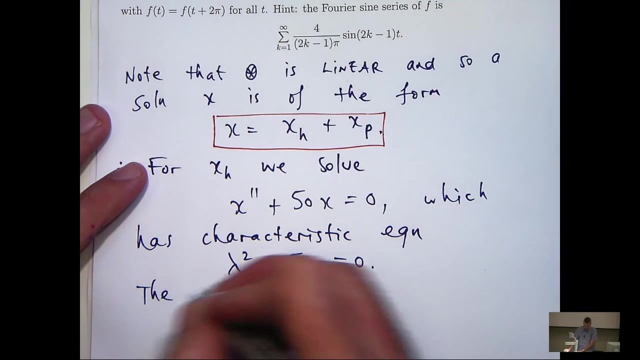 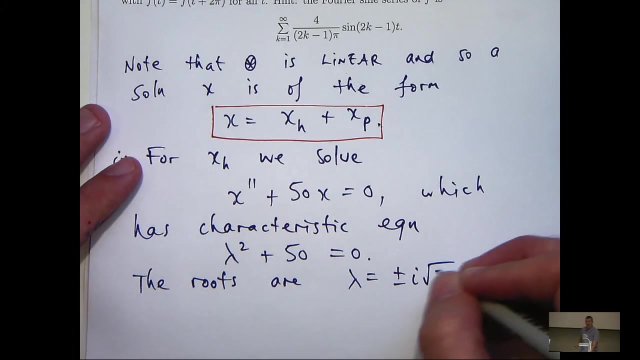 a quadratic- In this case it's lambda. squared plus 50 equals zero. Now this has roots: positive and negative, root 50i. Now I could write 5 root 5 here if I really wanted to, but I'm not going to do that. But 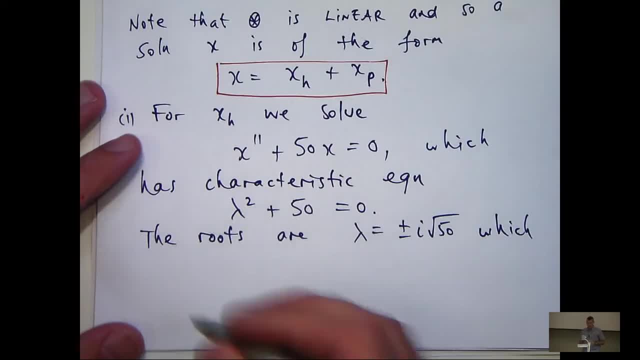 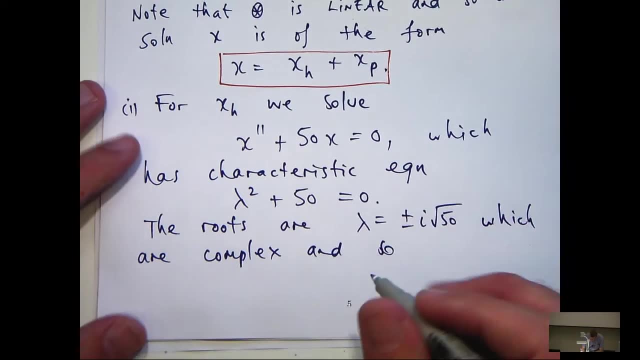 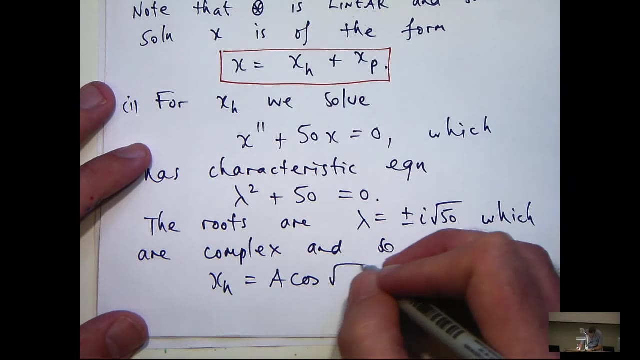 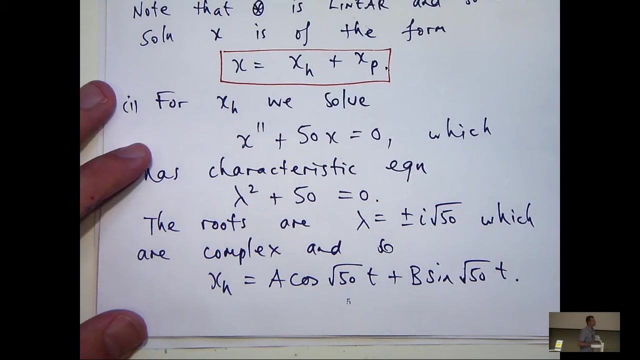 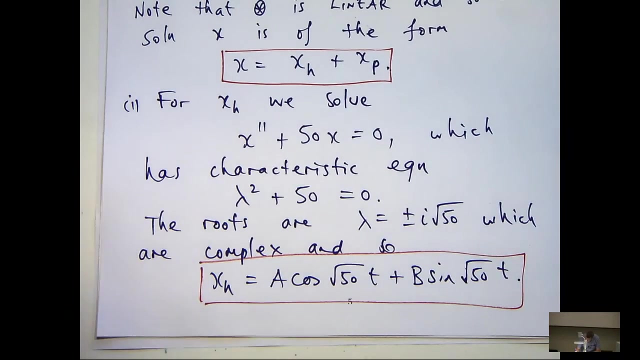 the important thing here is that these are complex valued roots And because they're complex, our x sub h has the following form: It involves cosines and sines. Okay, So that's the relatively easy part of this question: calculating the solution. 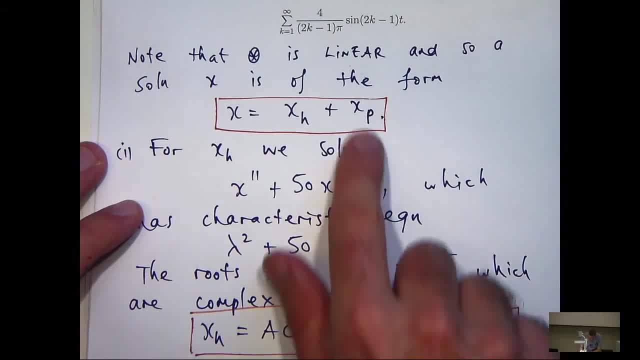 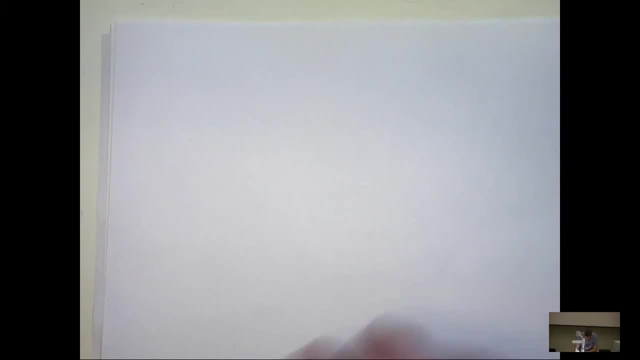 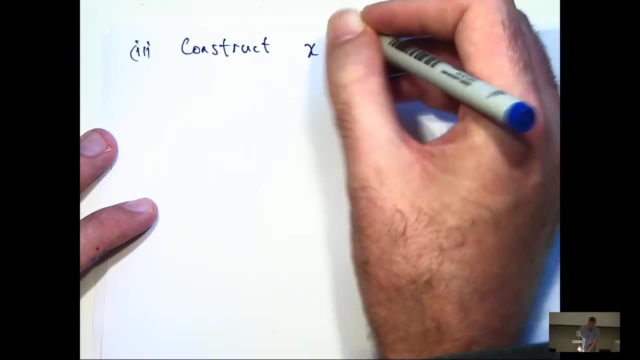 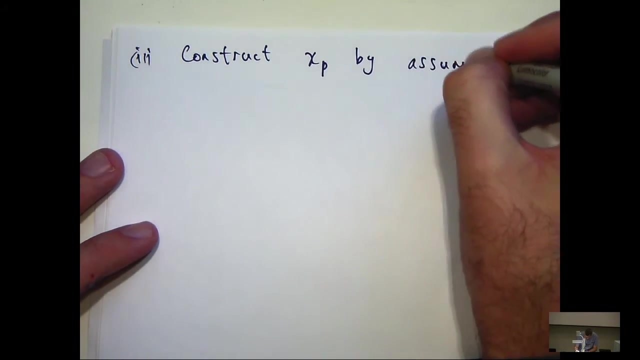 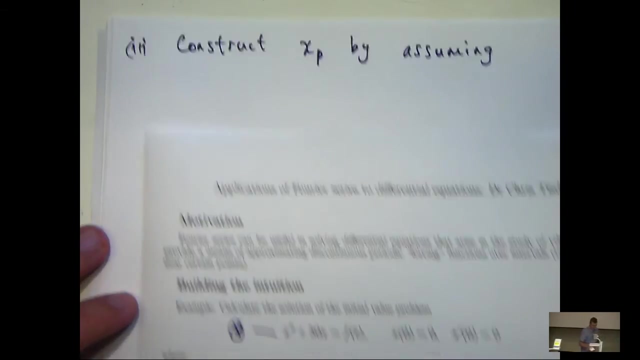 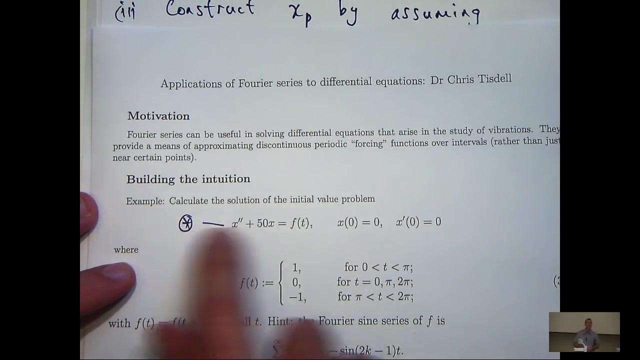 to the homogeneous problem, The more involved part is the particular solution. So let's have a look at that Now. we need to assume this particular solution has a certain form And if we look back to our original start equation, f of t has this form and f of t has this form. And so if 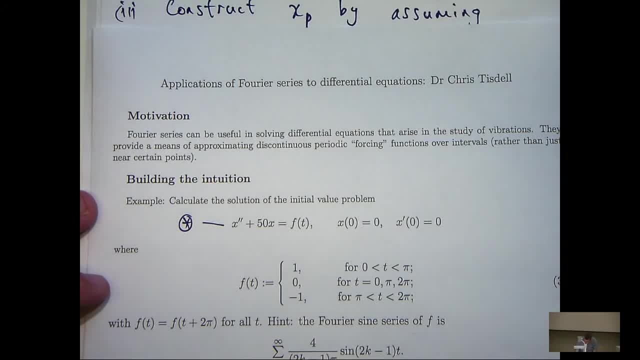 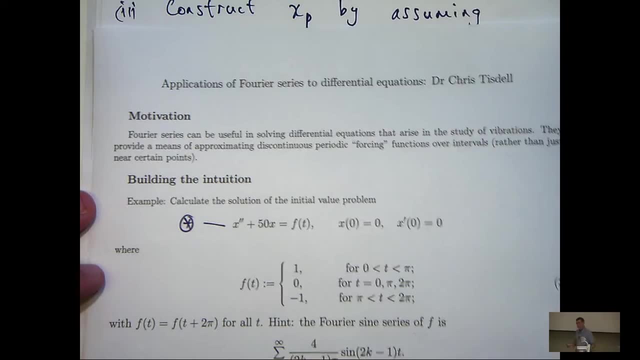 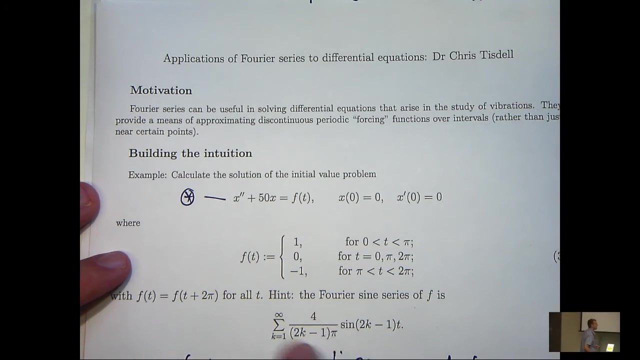 form and we know that the Fourier series will converge to this f of t, So I can actually replace little f of t with this Fourier series. So what I'm going to do is assume that our particular solution has this kind of form, just with a different coefficient here. So 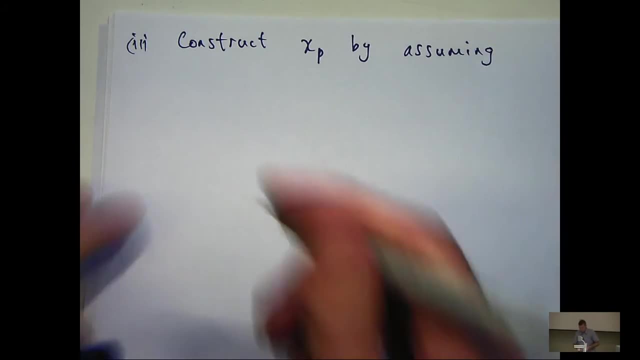 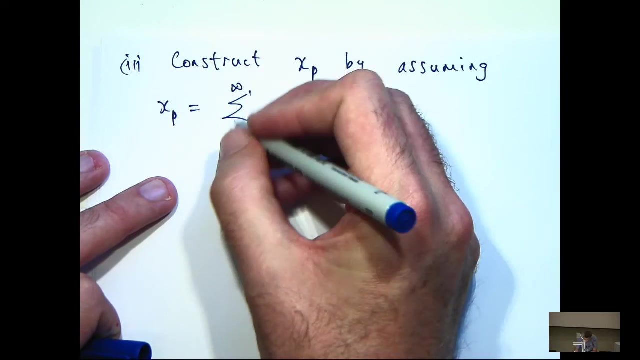 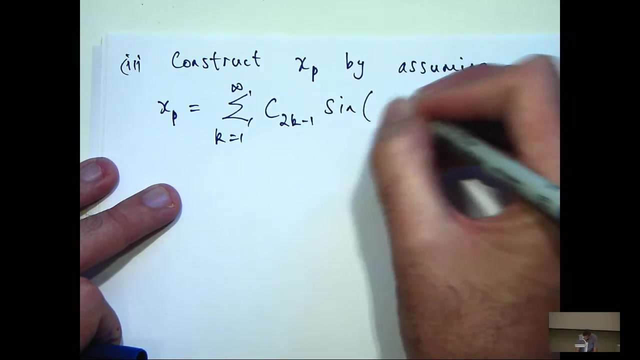 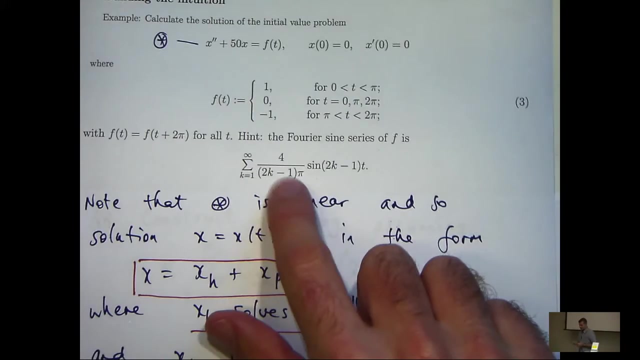 let me show you how I do that. So it's going to be a series that is similar but just with a different coefficient. So you can see in here there's 2k-1,, 2k-1, so I'm going to keep. 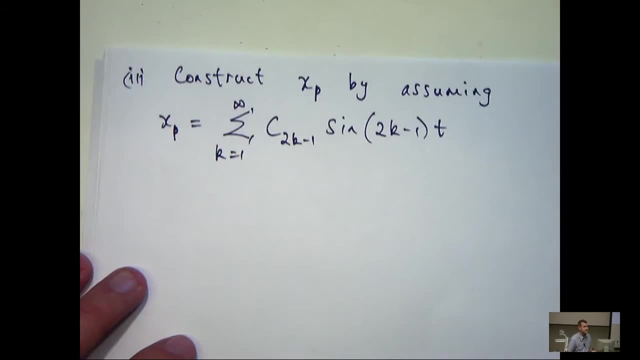 that with the subscript- and here also Subtitles- by the Amaraorg community. So what do I do? Well, I'm going to differentiate once, twice and sub this and its derivatives into my original start equation. That way I can calculate this coefficient, because once 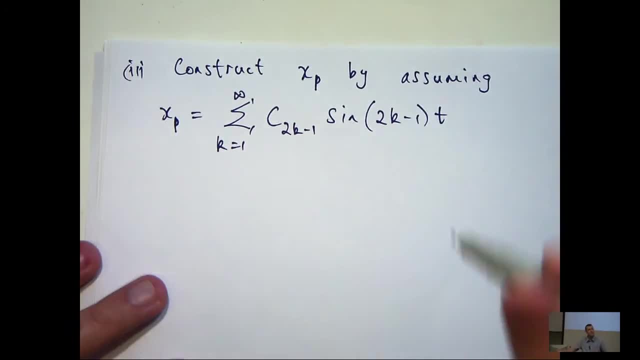 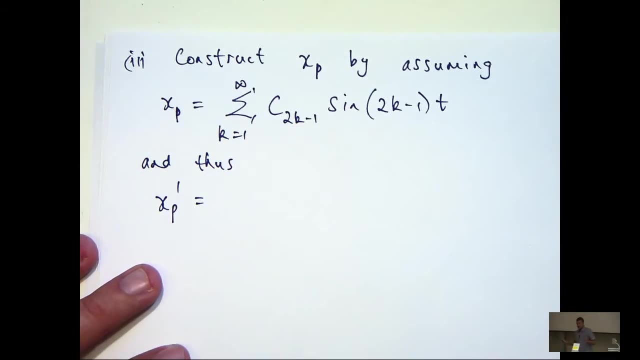 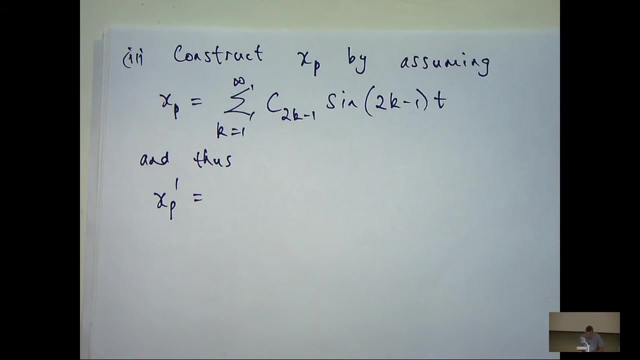 I have this coefficient, I get the whole particular solution. Now I'm going to make a big assumption here. I'm going to assume that I can just differentiate this and everything will be well defined. Now, the details of that is for another video, but at the moment I'm just going to assume. 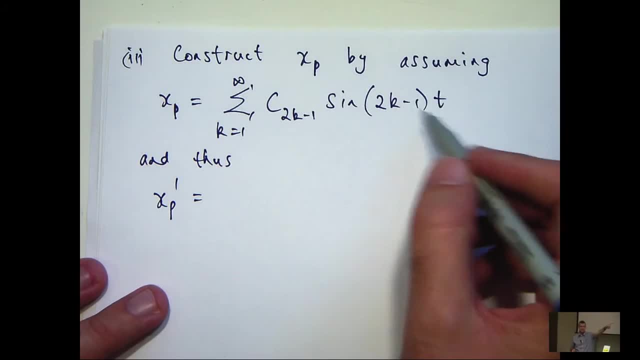 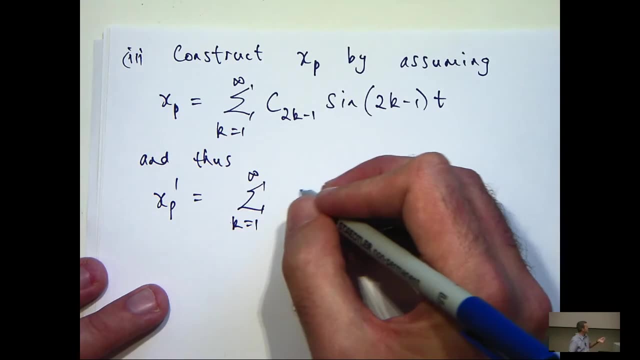 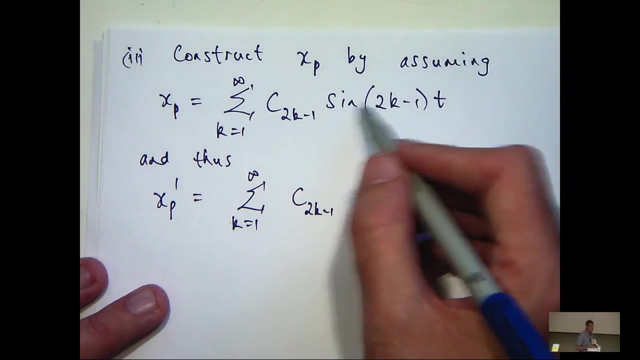 it and differentiate. So if I differentiate term by term with respect to t, I'll get something like the following: Subtitles by the Amaraorg community. Subtitles by the Amaraorg community. Okay, so this is going to come to the front. Sine will go to cosine and cosine will go. 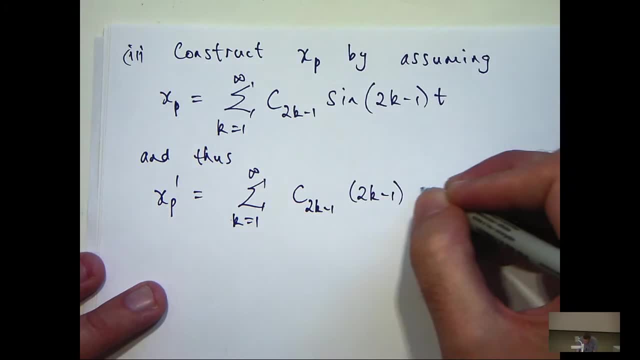 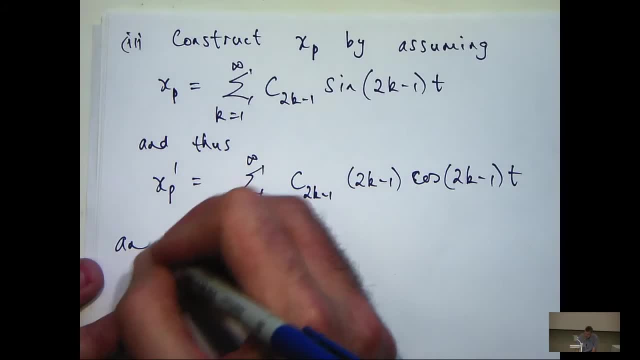 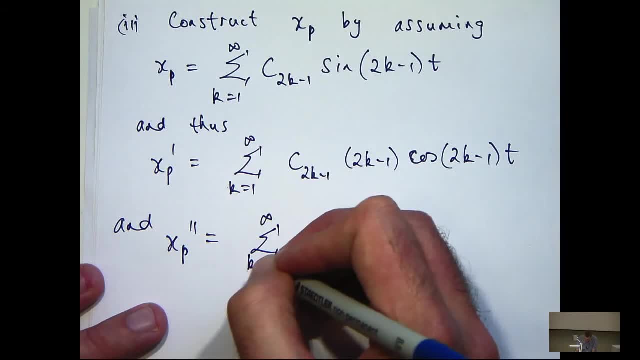 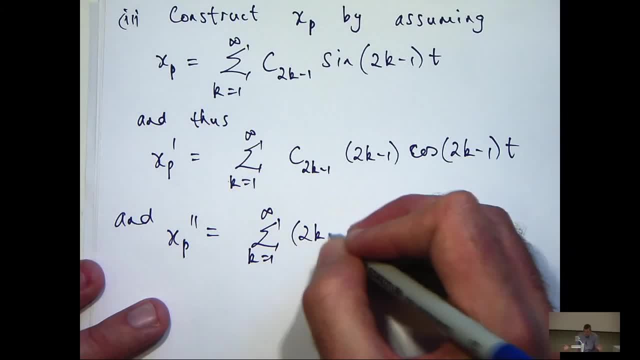 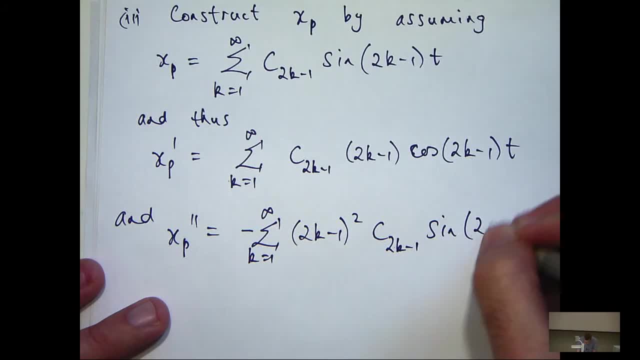 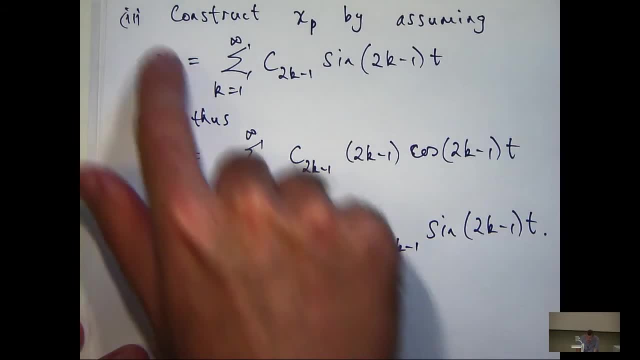 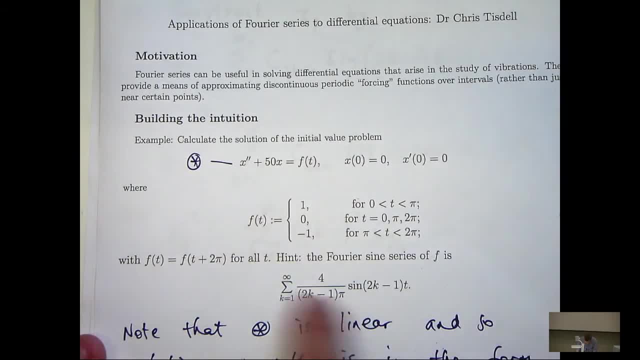 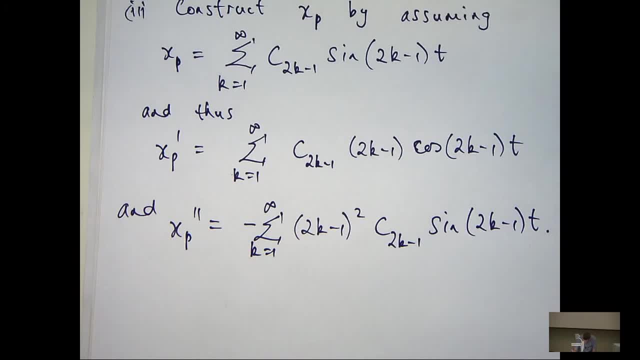 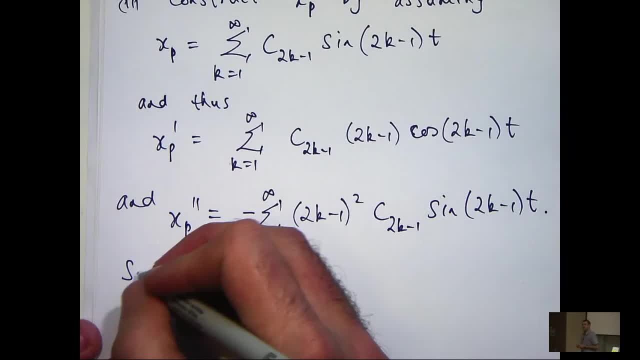 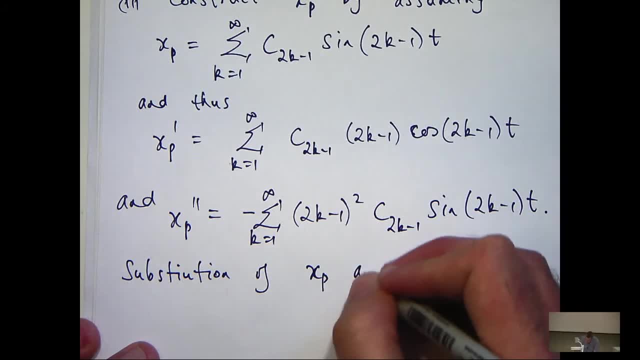 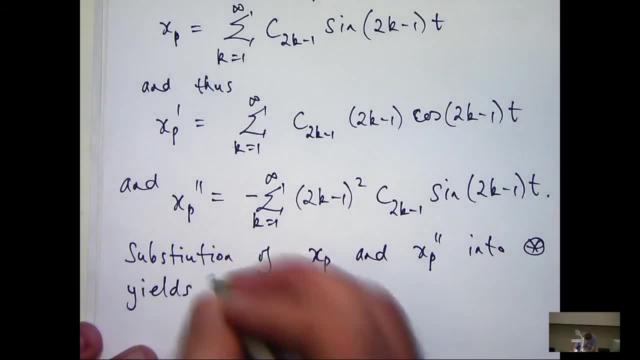 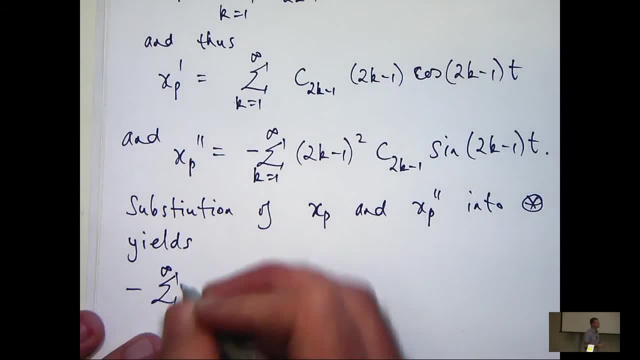 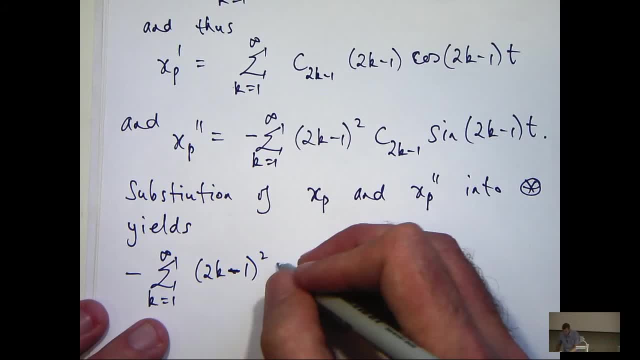 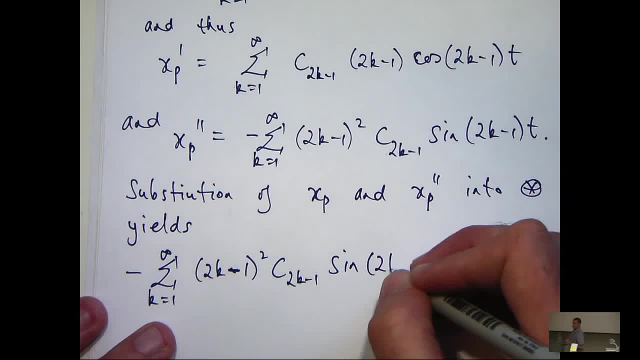 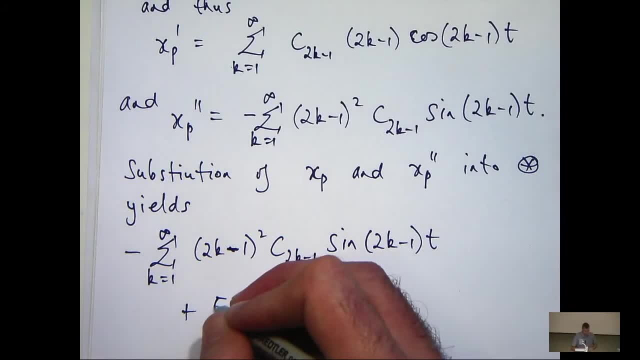 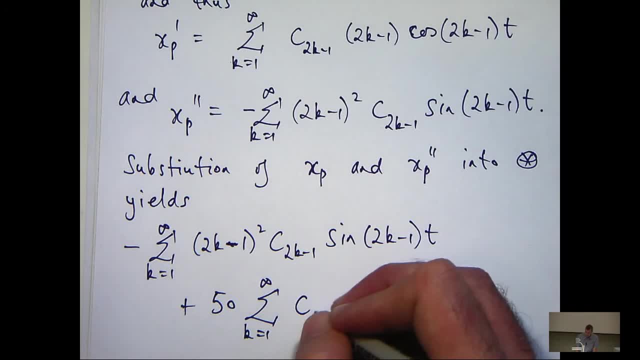 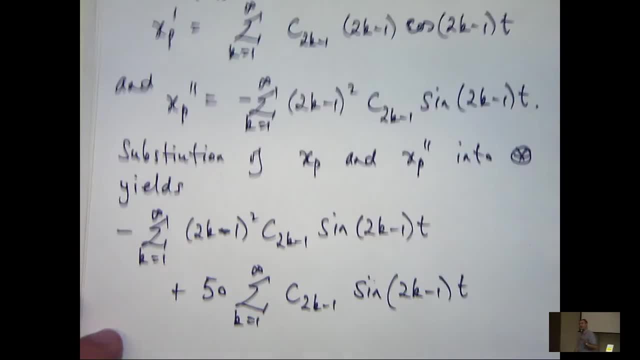 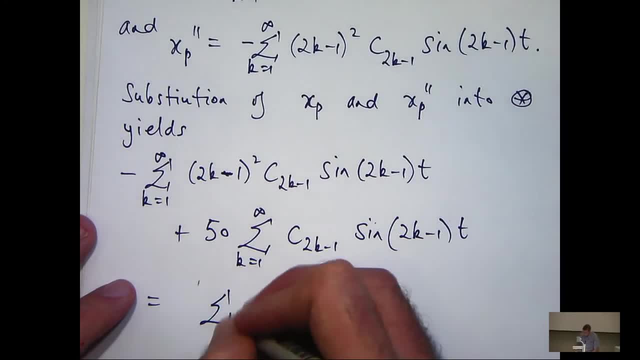 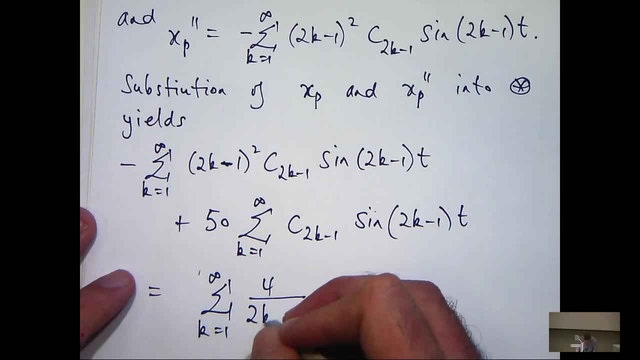 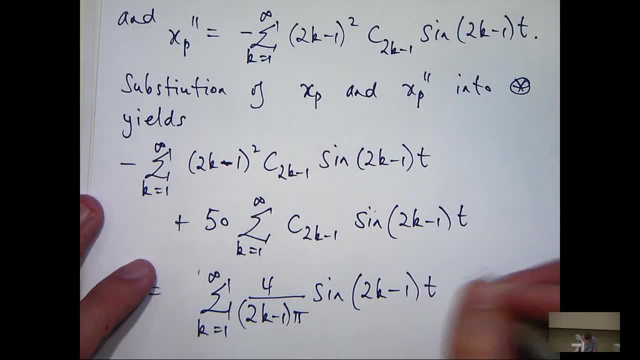 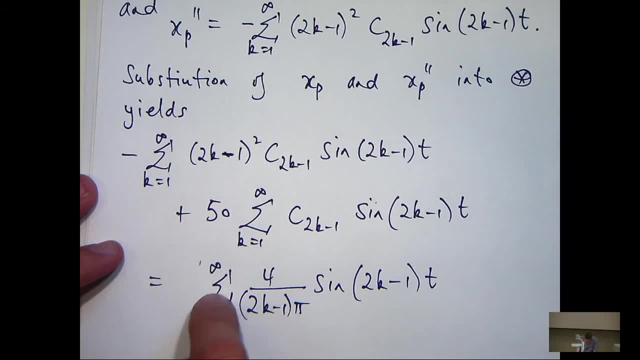 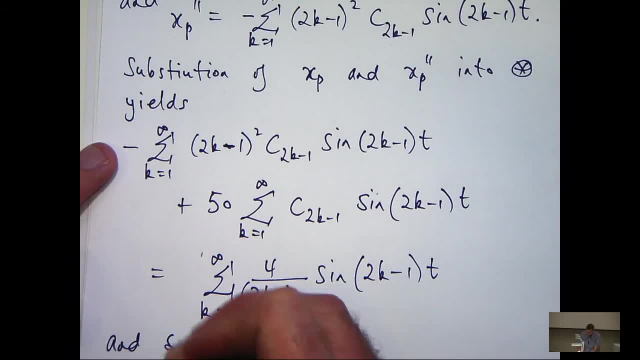 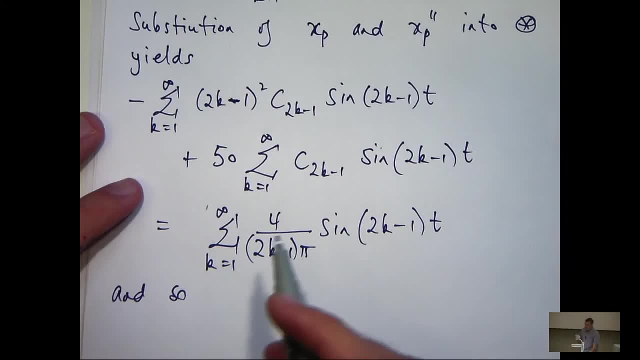 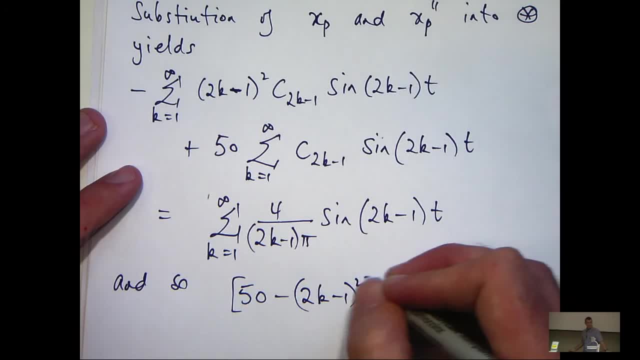 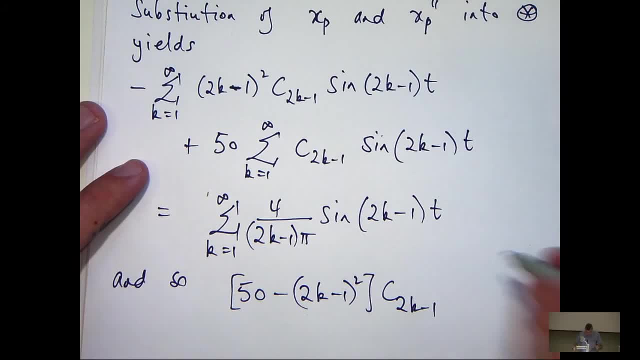 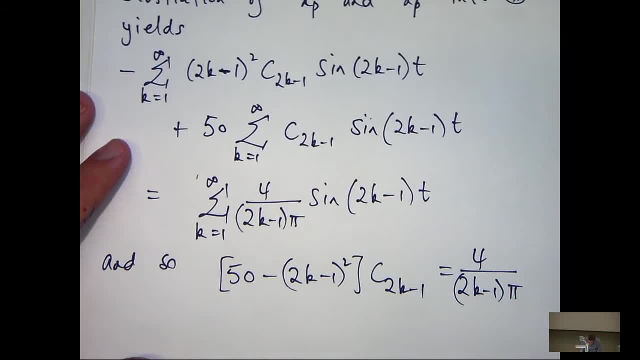 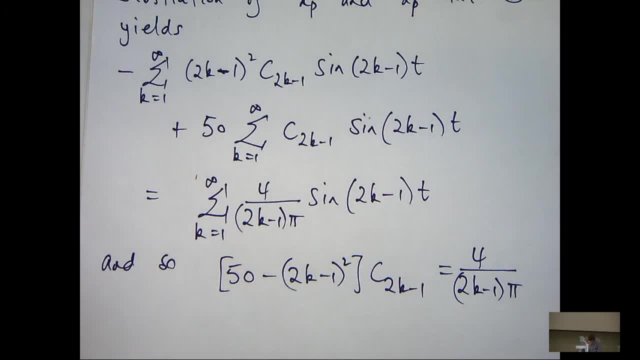 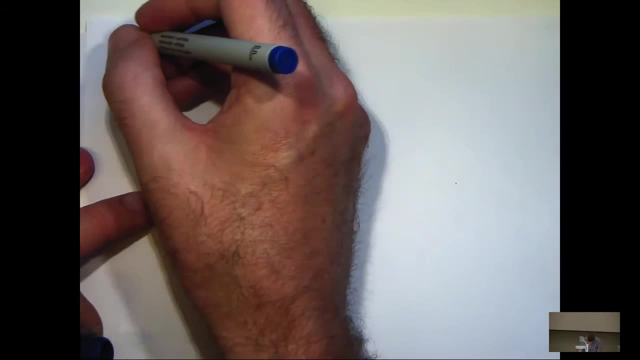 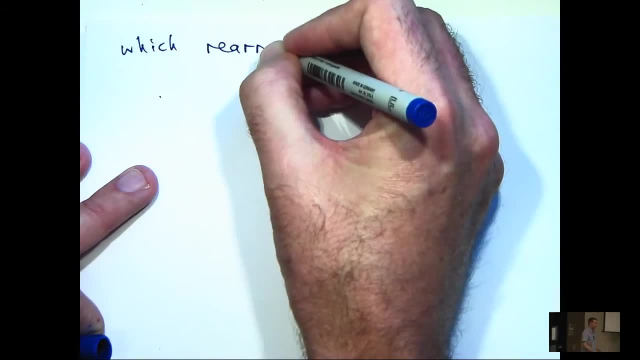 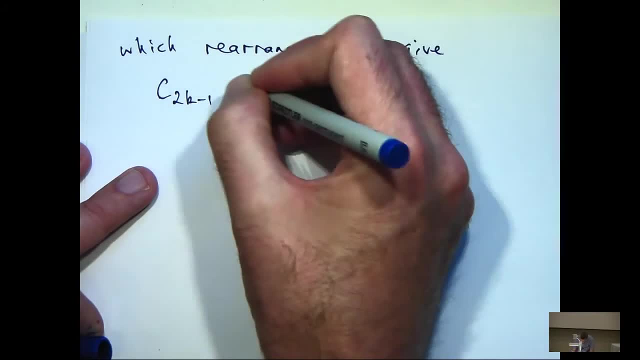 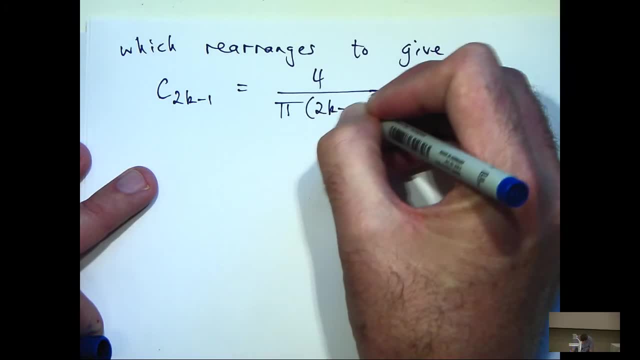 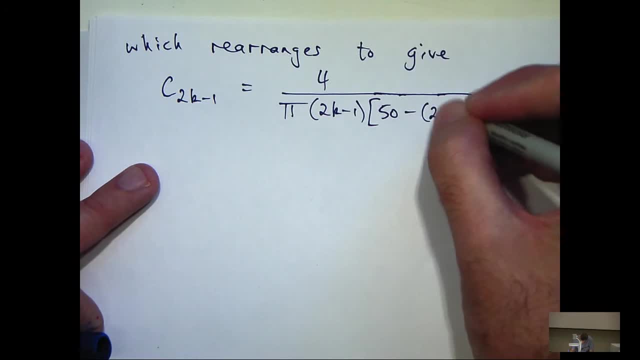 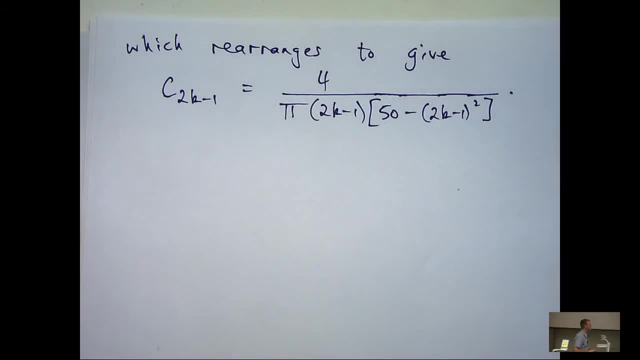 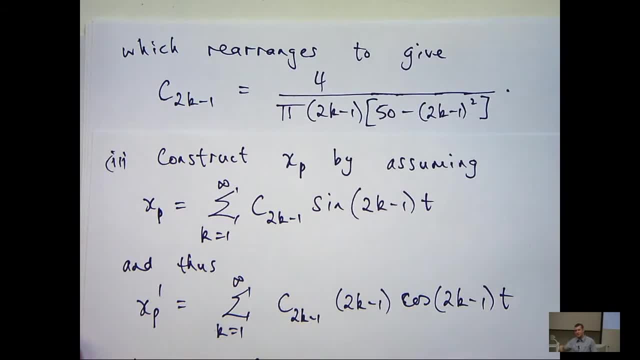 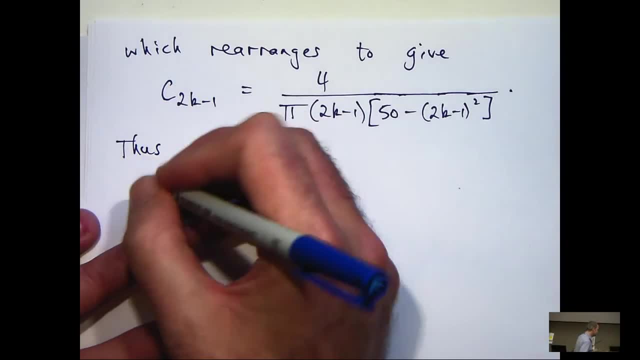 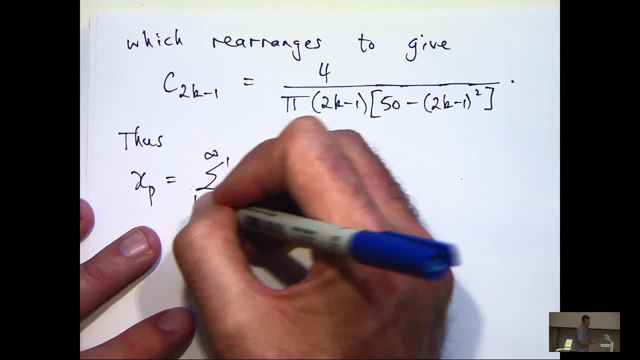 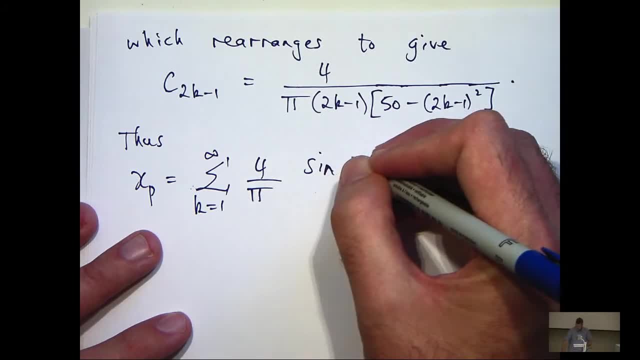 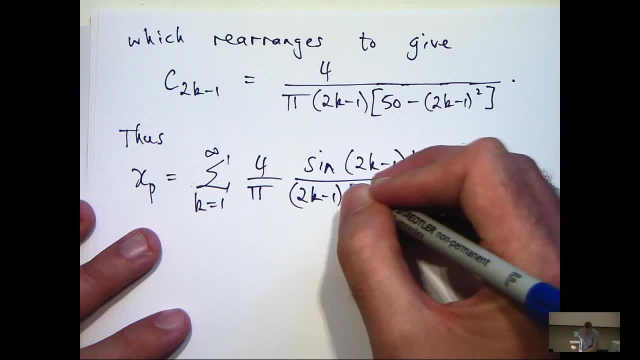 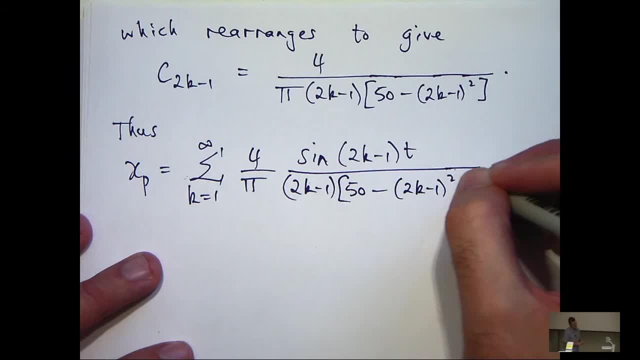 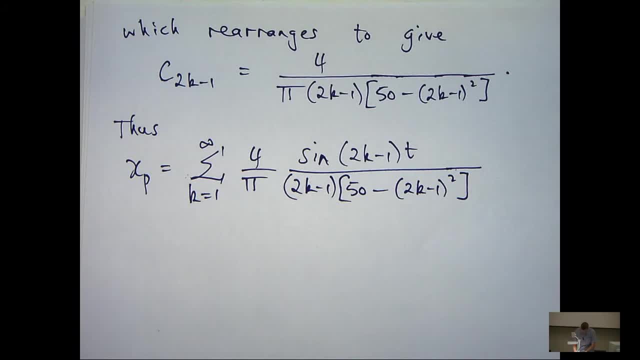 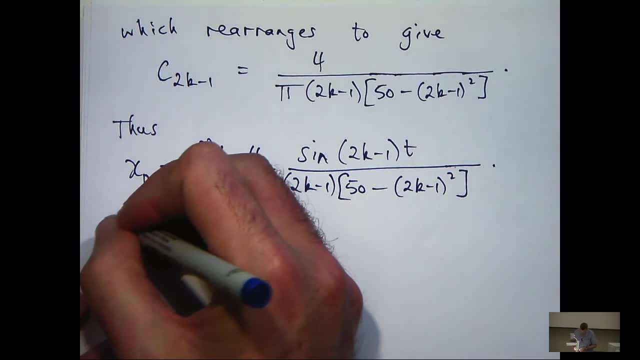 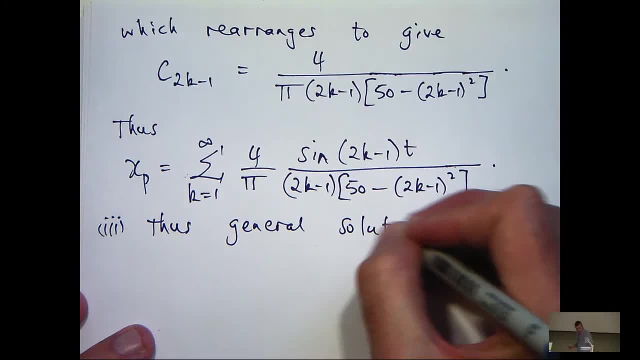 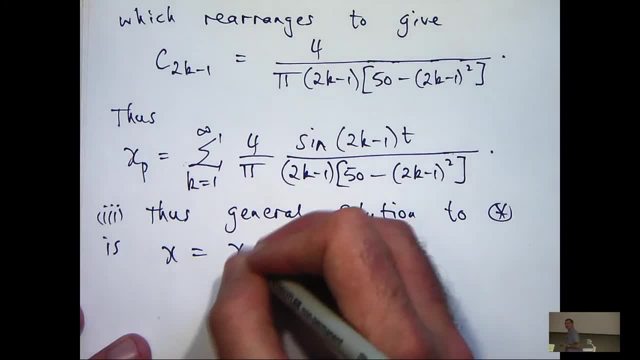 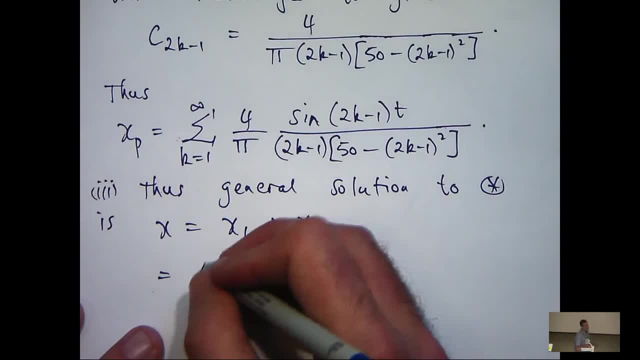 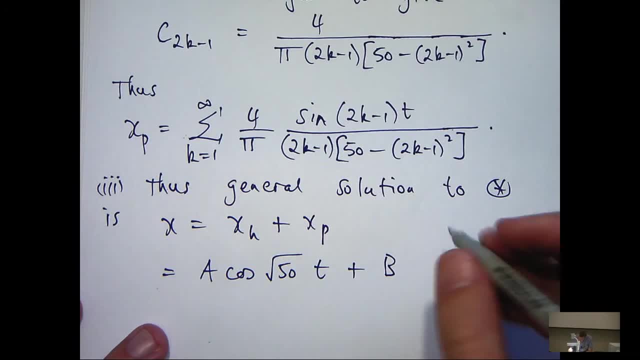 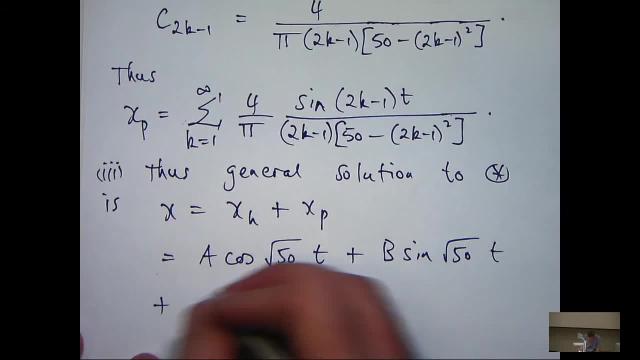 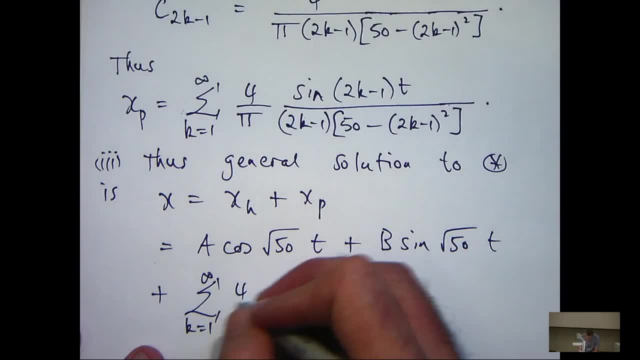 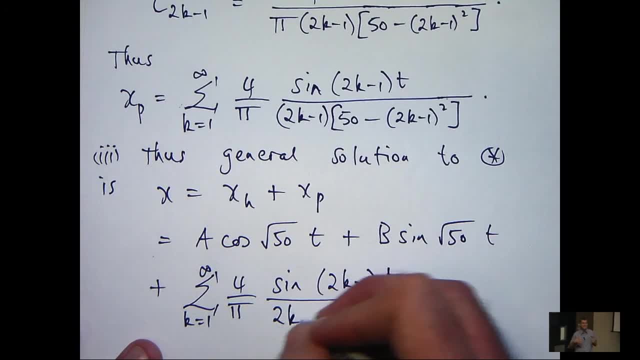 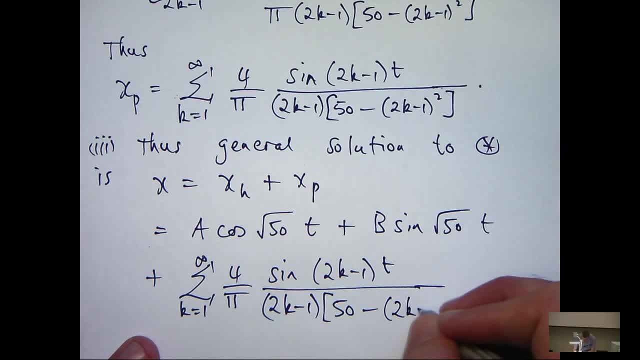 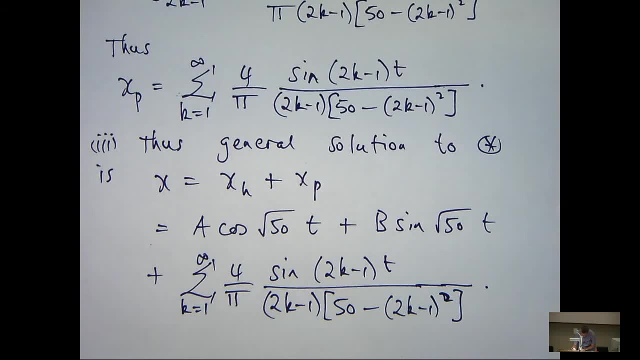 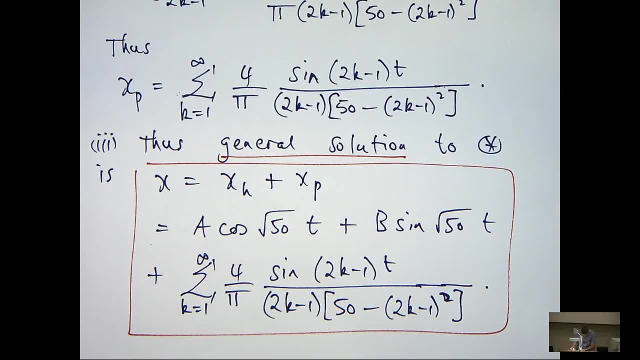 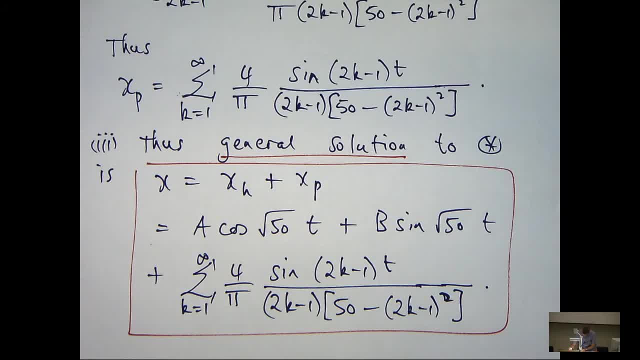 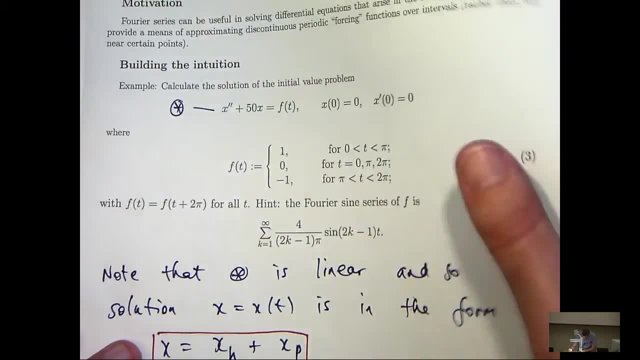 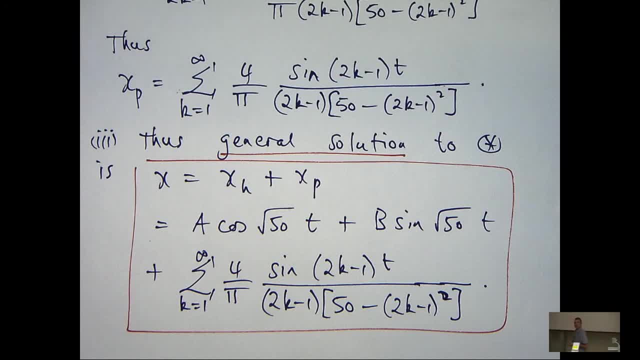 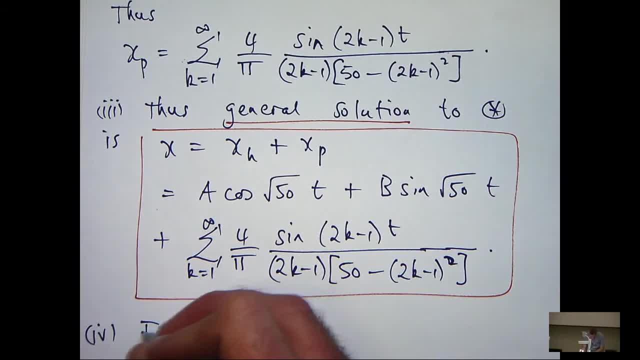 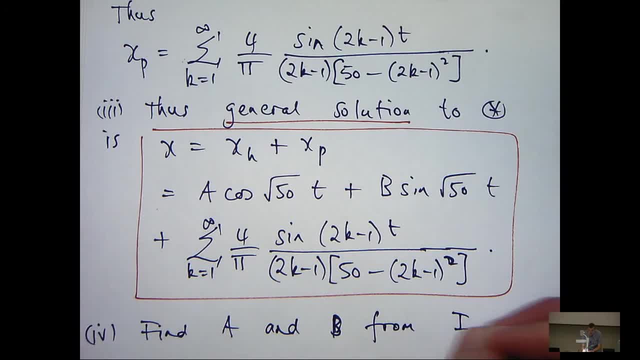 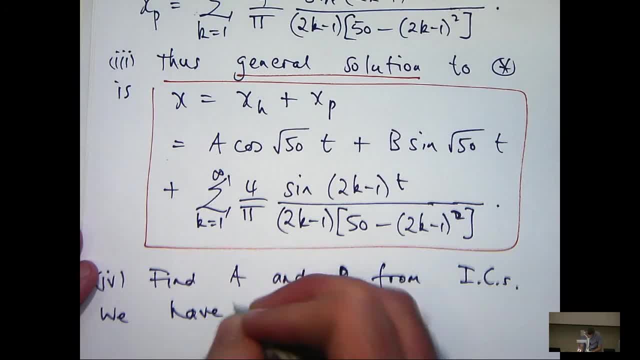 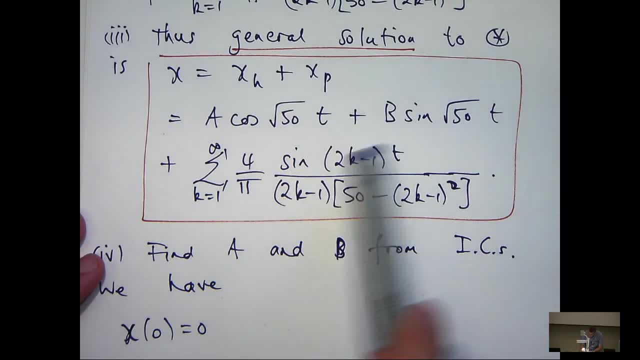 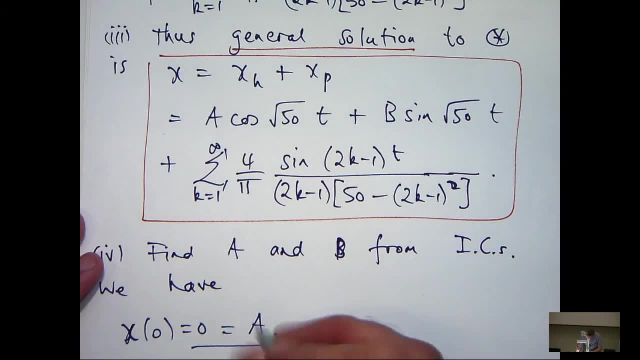 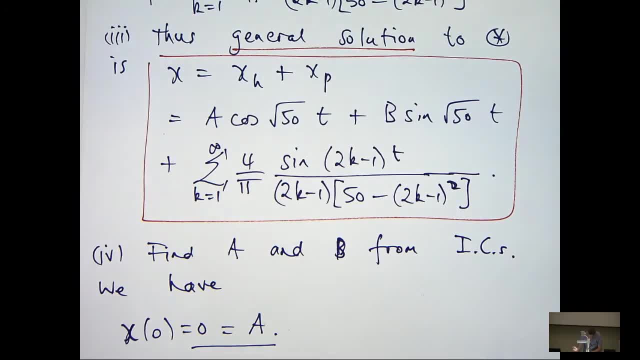 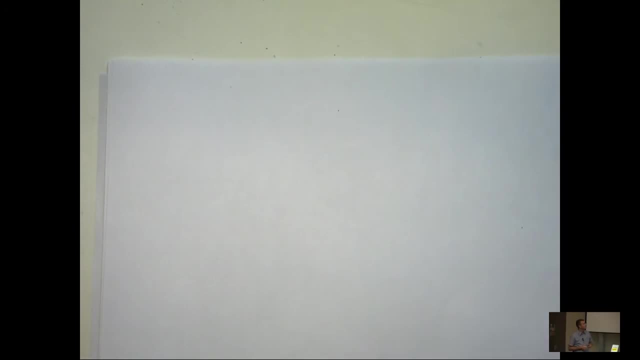 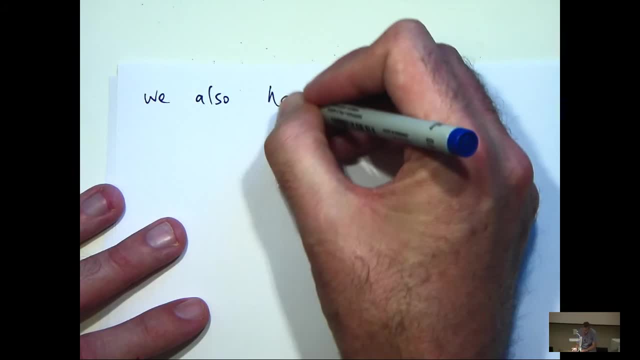 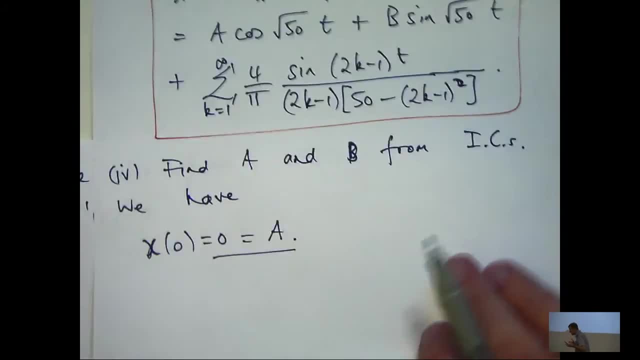 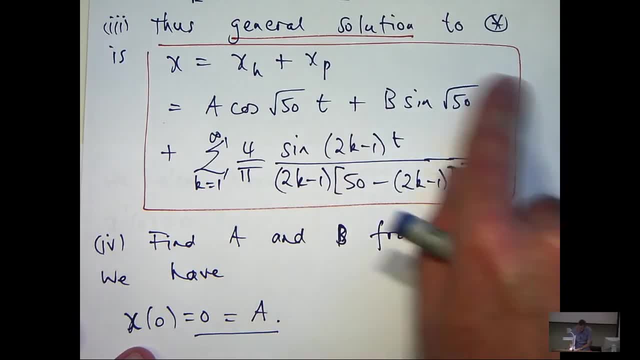 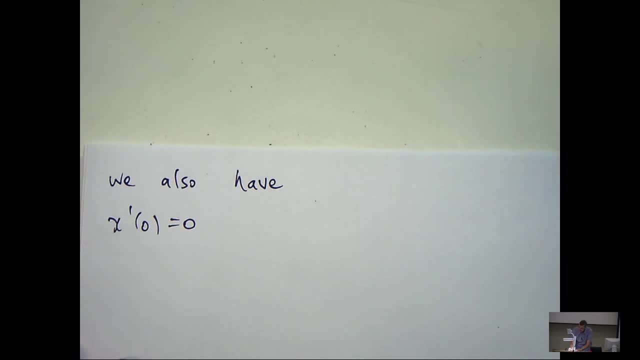 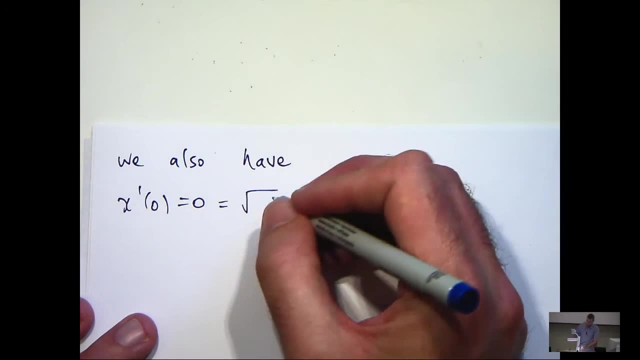 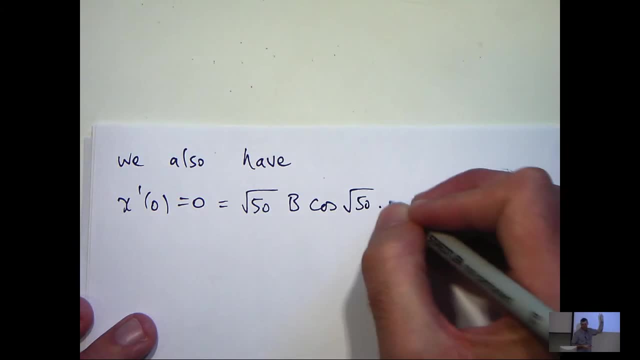 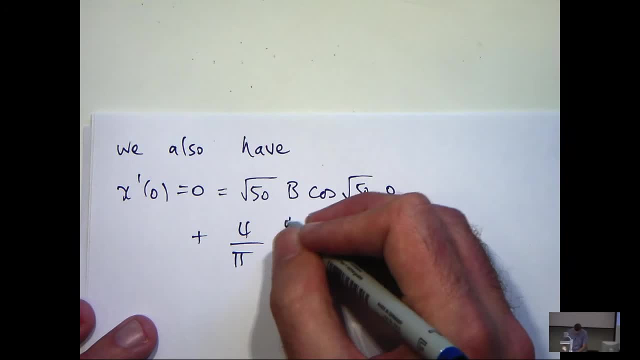 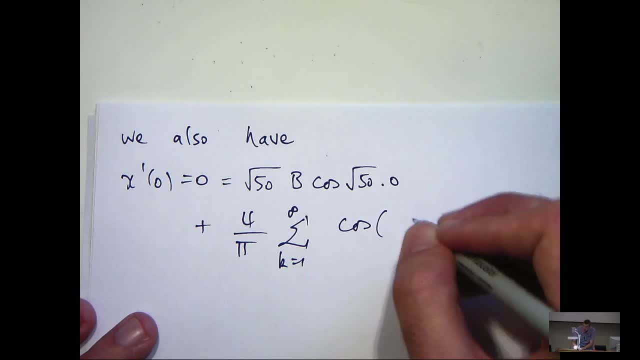 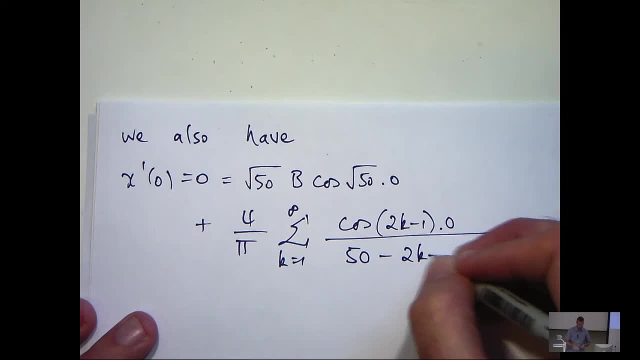 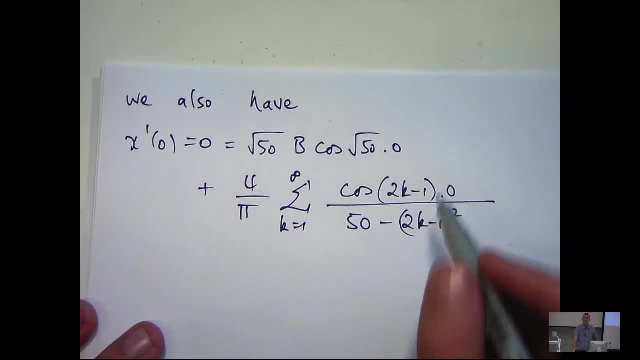 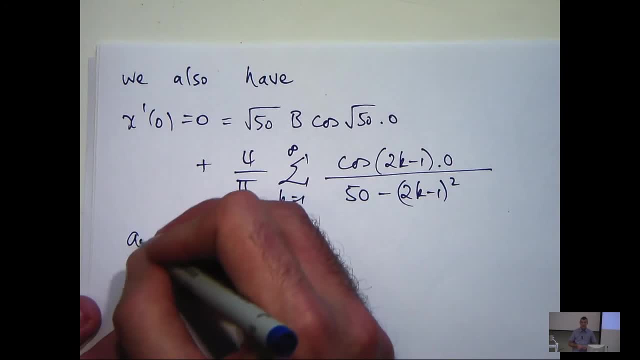 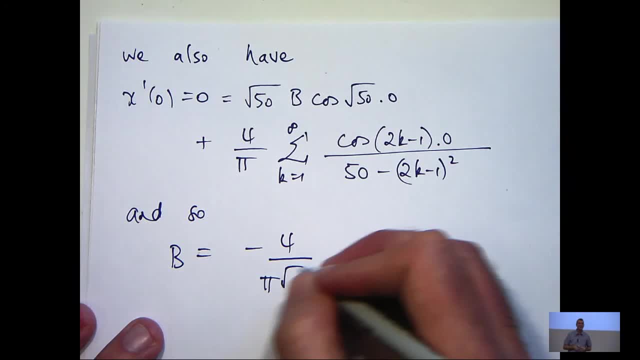 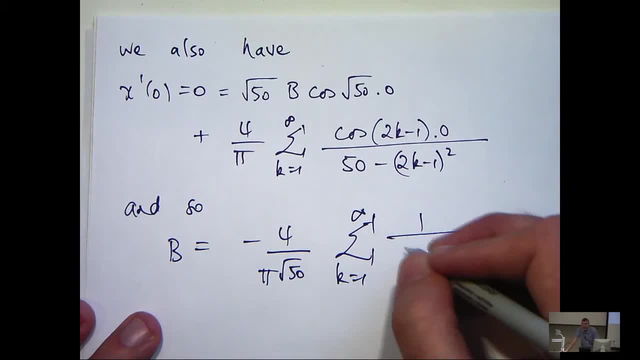 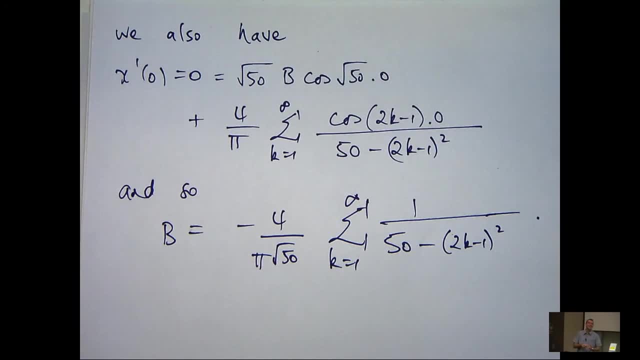 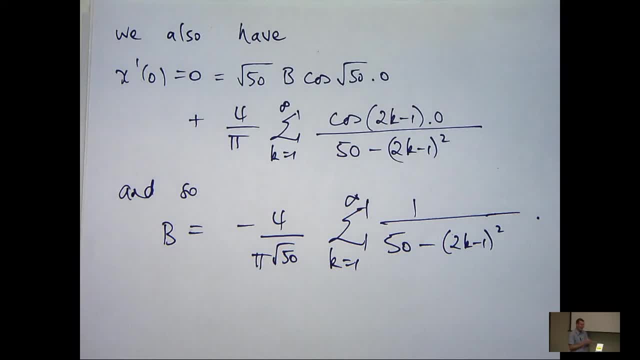 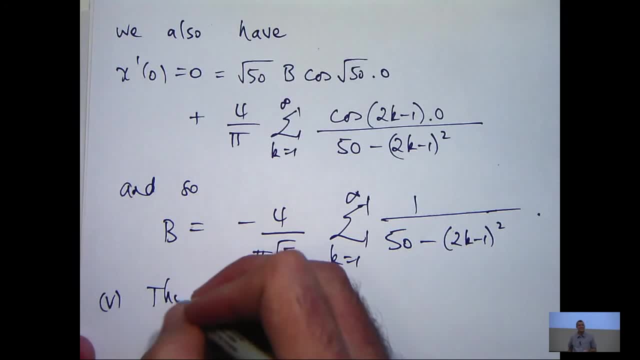 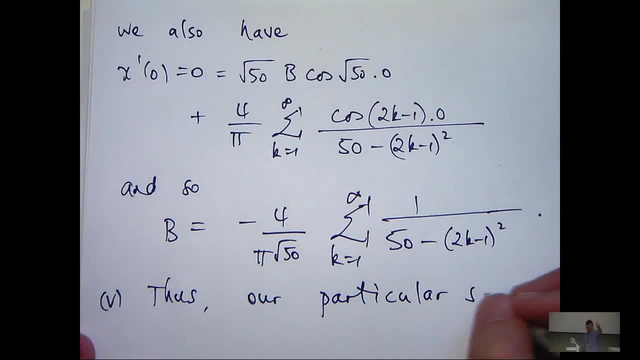 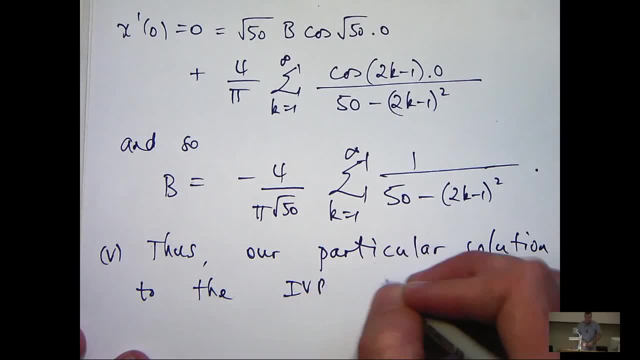 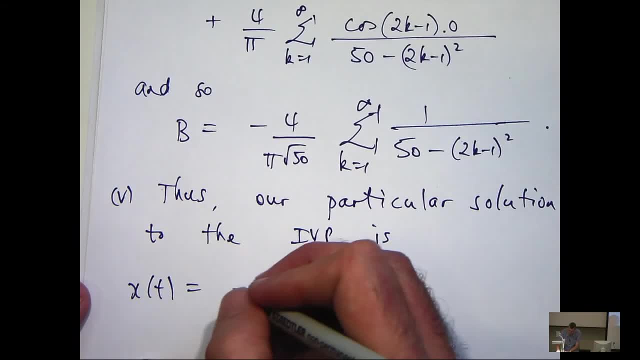 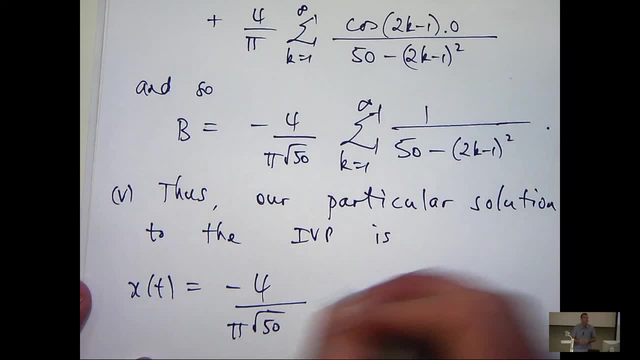 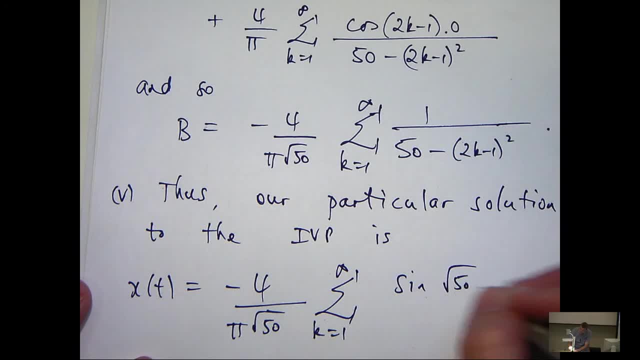 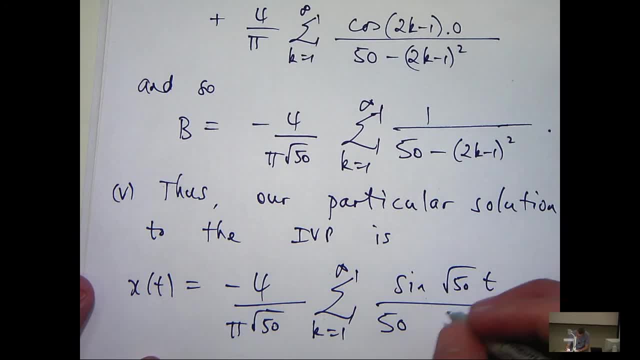 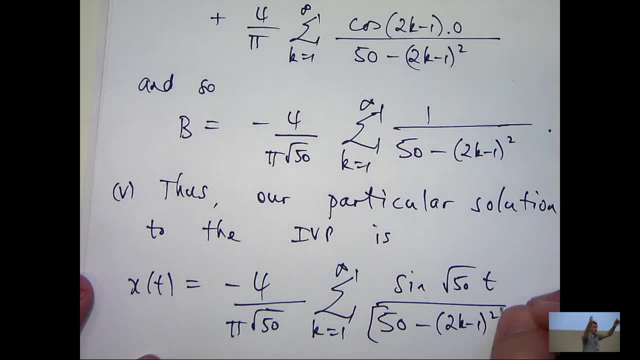 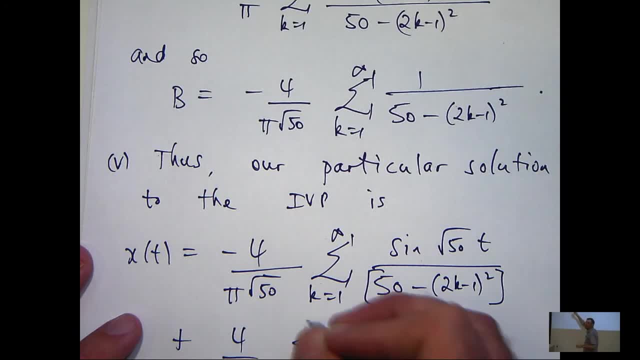 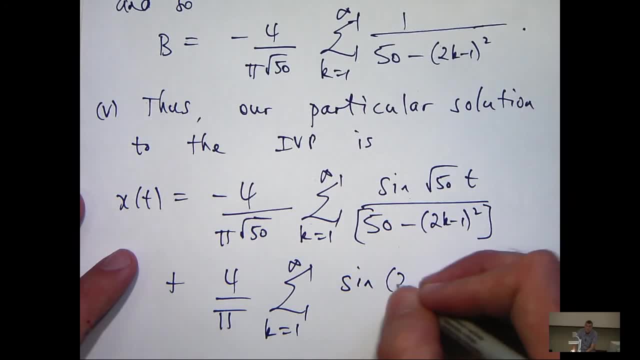 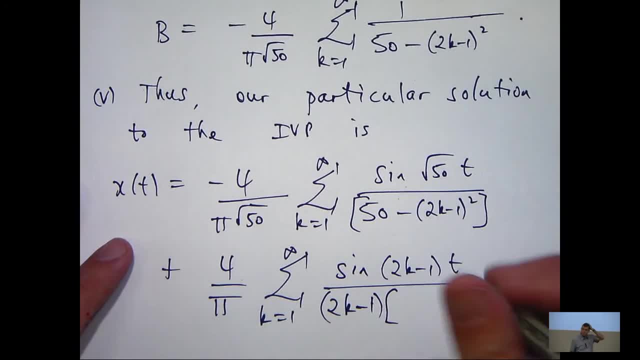 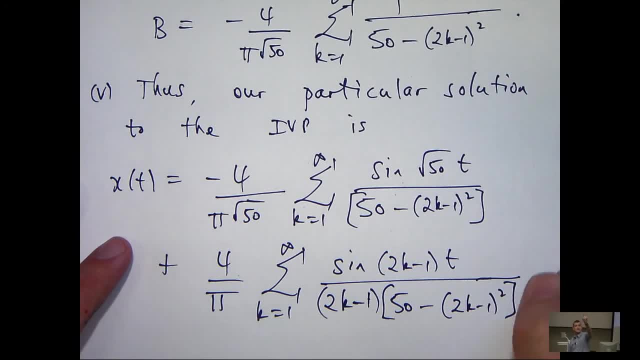 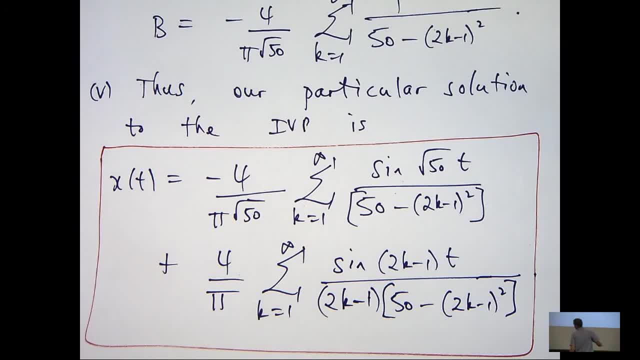 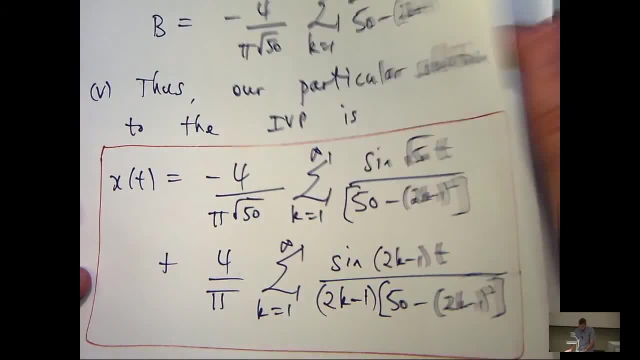 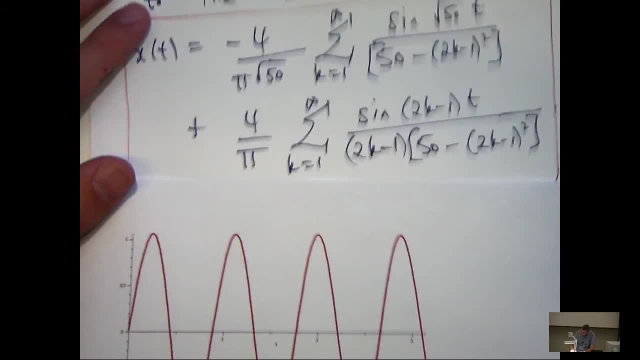 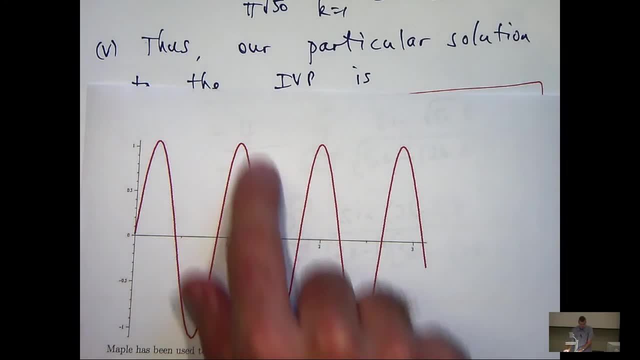 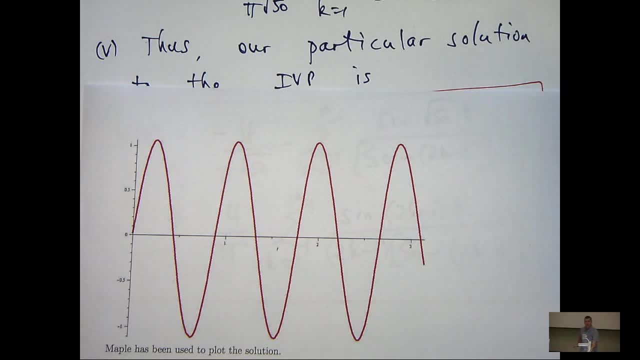 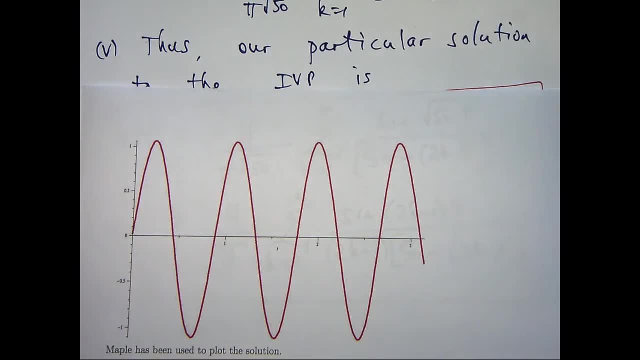 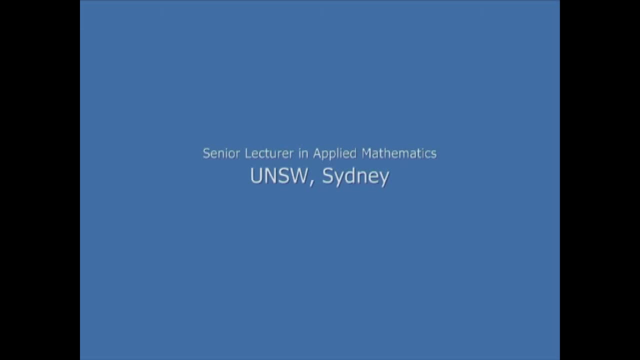